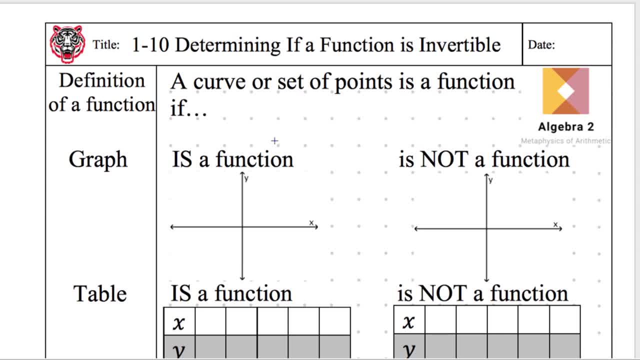 What is a function? Alright, Fiona. Yeah, there it is, If it passes the vertical line test. It's only slightly insulting. I know that Fiona had mammoth teachers for Algebra 1, and everyone else had me, and she was the only one that knew. 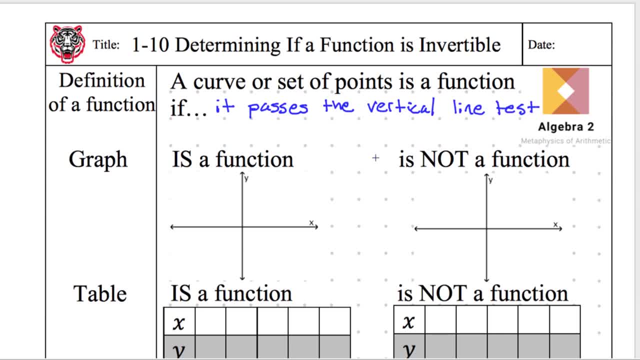 Which just means I didn't teach you guys and I feel bad about that. So what is a function graphically if it passes the vertical line test? So vertical line. by the way, if you didn't know a little bit of review, vertical line is a line that looks like this: 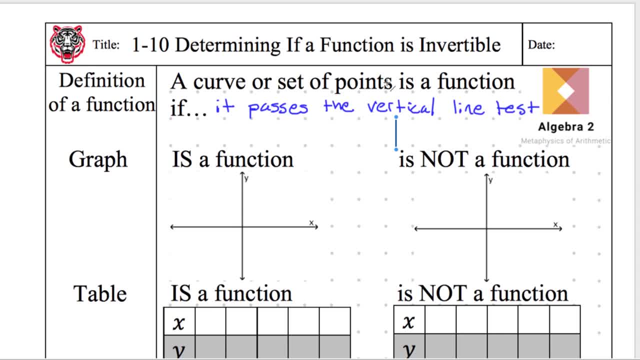 Boink. Oh, that's Try it again. Come on technology. There There's a vertical line. This is a horizontal line that I just did right there. That's vertical, So vertical goes Straight up and down. Vertical line test means I'm gonna draw that line and hopefully it only passes through once, through the function or the curve or the set of points. 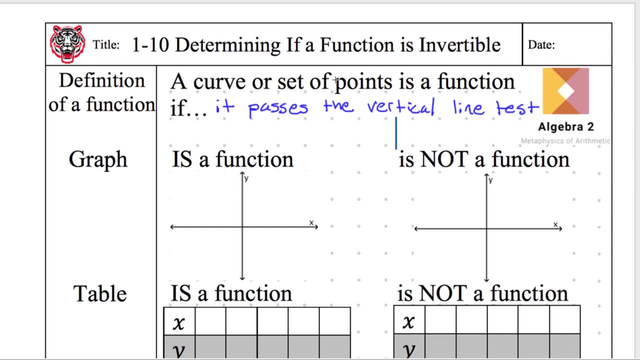 So let's draw something, that is a function. If I have a straight line, that's a function. If I have a quadratic graph, that's a function. Let's just go ahead and draw a straight line. That's pretty straightforward. 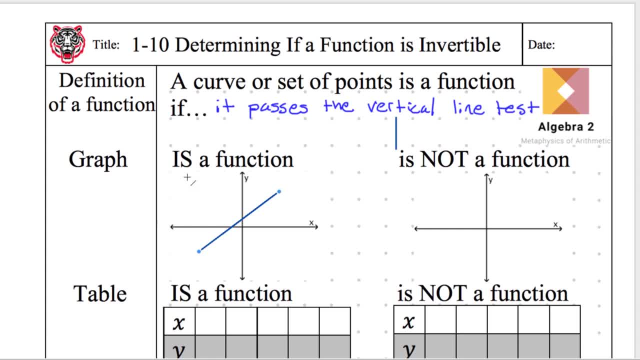 Let's draw a straight line that looks like this Boink. That's a function. Here's why This is a function: because if we draw a vertical line through every single possible x coordinate, there's no way that I can intersect this function more than once. 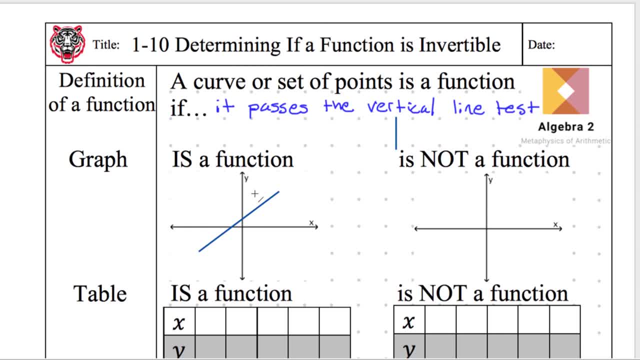 See, here I go, Look, Oh whoops, I don't want to change that color, I want to change my new color. If I draw my vertical line, it only passes through, And you're drawing this on your own notes as well. 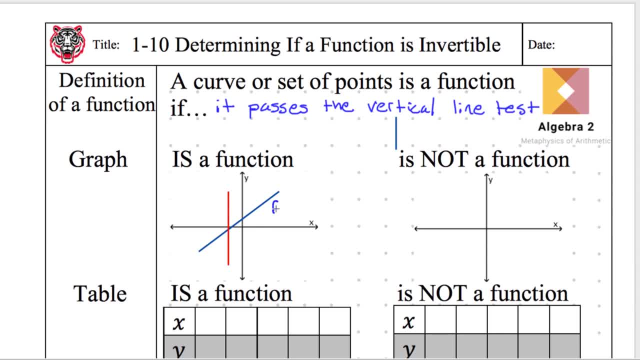 It only passes through my original blue function. I'm gonna say my blue function was my f of x. It only passed through my function once and it was at this point. It didn't pass through it twice If it passed through it twice thrice. 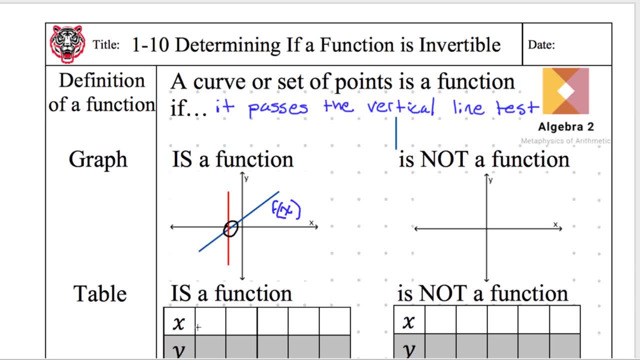 I don't know what four is. Any times more than once it'd be a vertical line: one, two, three or four times. that is not a function. Let's see something that is not a function. Here we go. 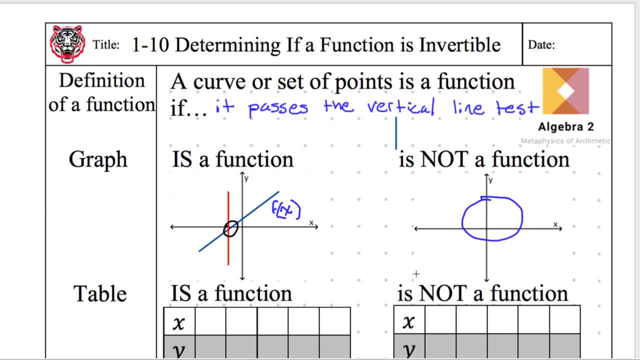 This is not a function And I have technology so I'm gonna make my nose look really nice. That's not a function. Excuse me, Someone explain to me why this is not a function. Why is a circle not a function, James? 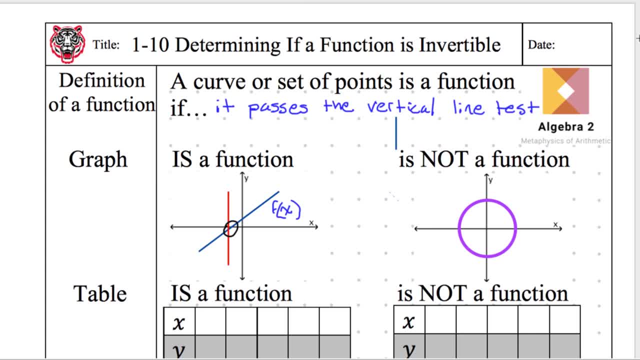 If it goes through twice, What goes through twice? A vertical line? Yeah, so if I draw a vertical line almost anywhere, in fact- Oop, I'm still on line mode, Go backwards, Mr Sandell, If I draw a vertical line, it goes through it twice. 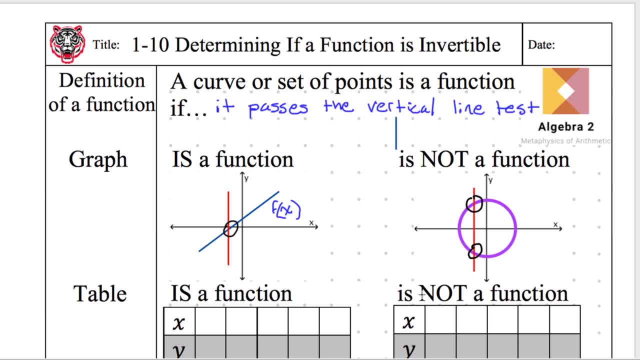 You can see it. it's clearly like: right there, right there, It goes through it twice. It does not go through it twice, It does not pass the vertical line test. Therefore, it is not a function. Everything always builds on top of each other. 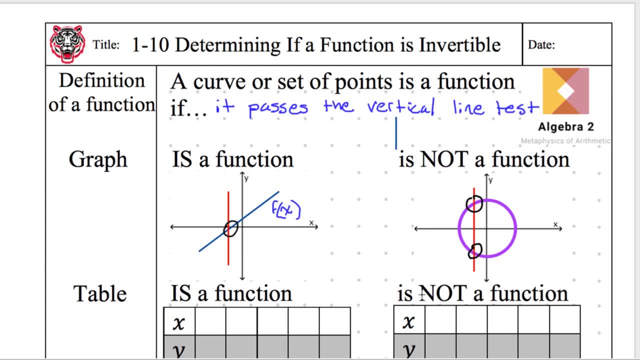 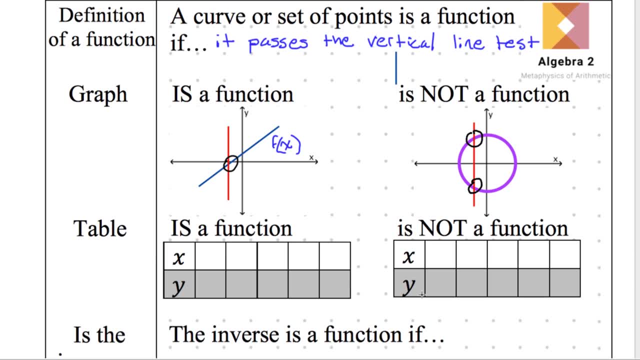 Hopefully you have mastered vertical line tests. You're reviewing it now and we're going to apply this to tables, and then we're going to inverse functions. All right, so let's do a table. that is a function. So my values I'm gonna choose are: 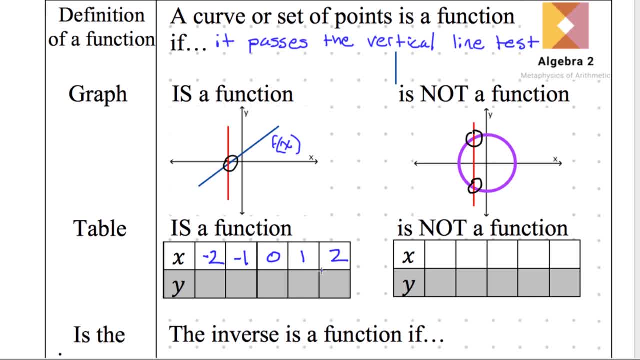 negative two negative one, zero, one and two. We're okay girls. Yeah, Okay, Kiana's snuggling with Stego- They were great, Okay. so this is a function. Let's choose something like five. 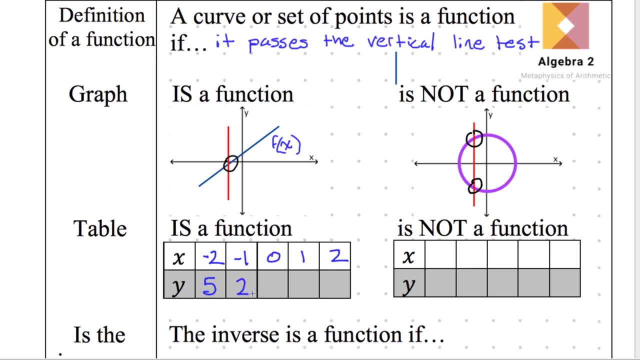 something like two, one, two, five. That's a function. And here's why, If I were to draw a vertical line through these points, that vertical line would never hit the same point twice. This coordinate pair is a point. That coordinate pair is a point. 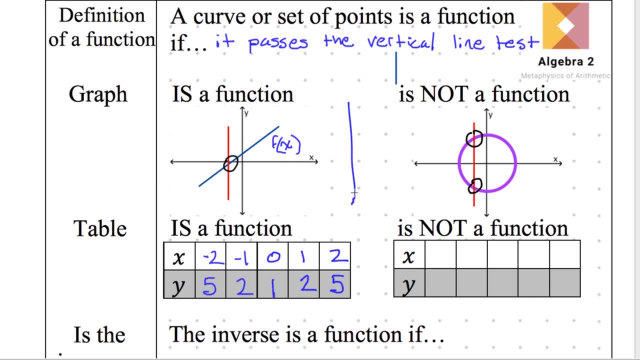 If I were to graph all of these points and drew a vertical line, I would never be able to cross more than one point at a time. That's the reason that this represents a function. Here's an example of something that is not a function. 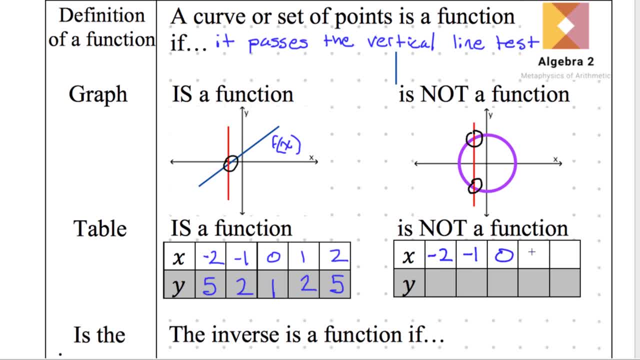 I'll do my same points: Negative two, negative one, zero one and two. Actually, sorry, I have to change that, Bruh. why Let's change this to a negative two? because otherwise it's not gonna work. 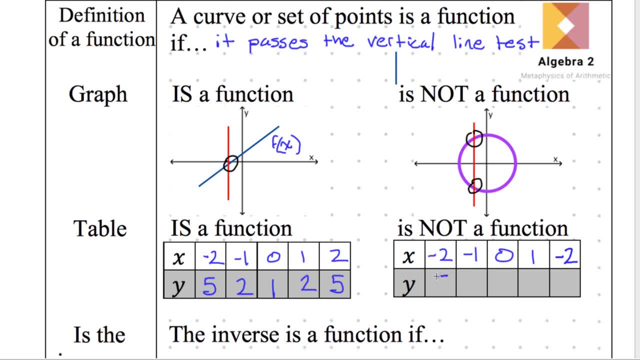 Bruh. All right, so let's change this to negative: two, five, two, one, two, three. All of a sudden, this is now not a function, And here's why Hold on, I'm gonna pause. 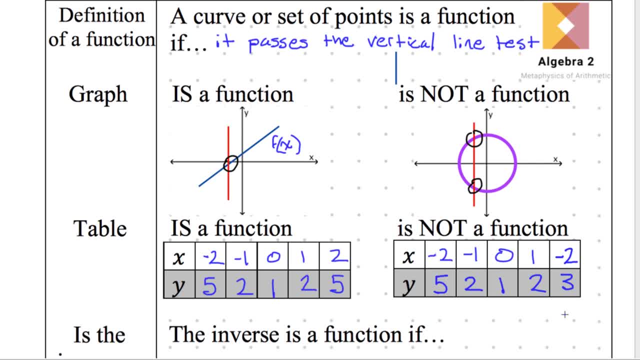 because people are still writing this down. This is not a function, because if I graph this point and this point, I can kind of just sketch it on this graph up here. If I graph negative two, five, that would be somewhere like right here: 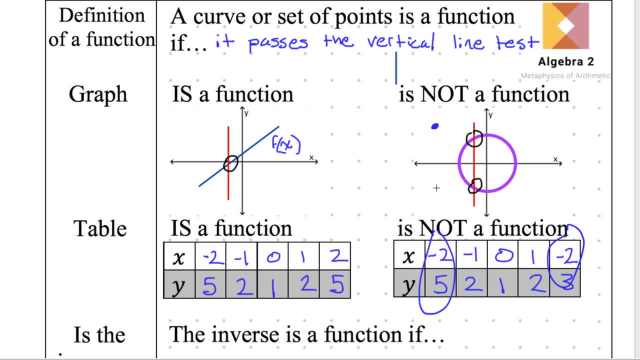 Maybe I'll do it like out here And negative two, three. I go to the same x coordinate but a different y coordinate. If I have two points on top of each other, if I drew a vertical line it passes through both those points. 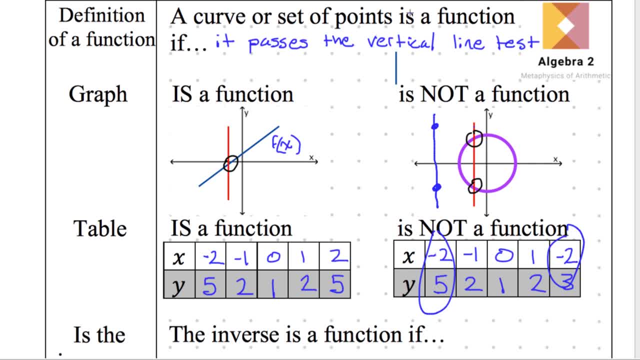 This is no longer a function. So far, so good. Everything is coming from Fiona's definition. It passes the vertical line test. That's the only definition that you need to know to know if something is a function, It applies to tables. 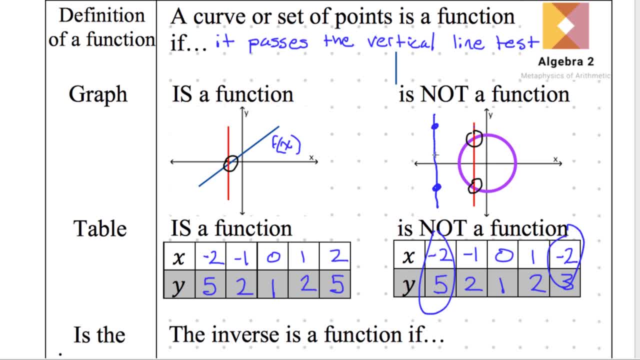 It applies to graphs. It can apply to equations, if you know what their graph looks like. In fact, you can use equations a bunch of different ways, but that's the general idea. This is not a function, because we have two points. 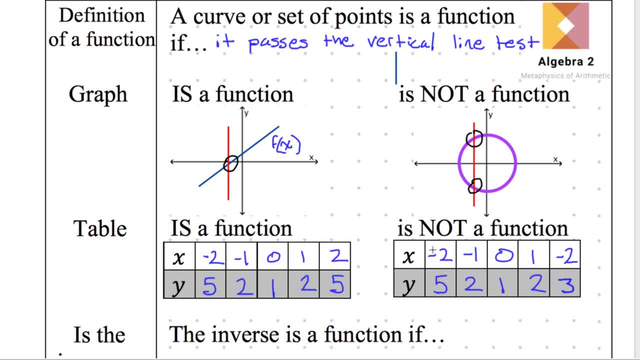 two values for the same x. That's another way of saying it. Two values for the same x, That is. I am a computer. I will always give one answer: Plug in negative two. what do you get? Oh, I'm stuck. 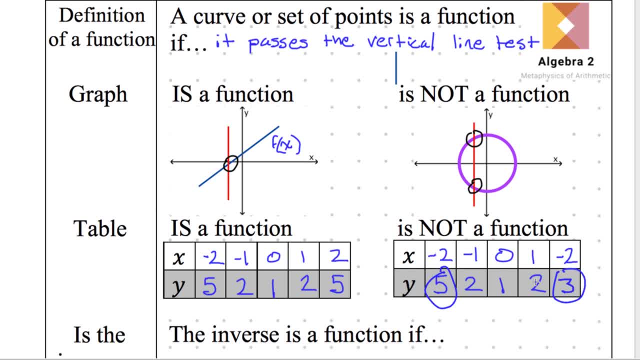 I don't know if I should give you five or three. I can't give you two answers. A function can only give you one. I don't know. should I give you three or five when you give me negative two? I'm not sure. 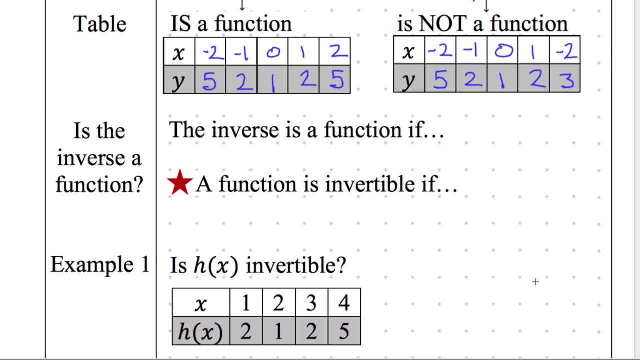 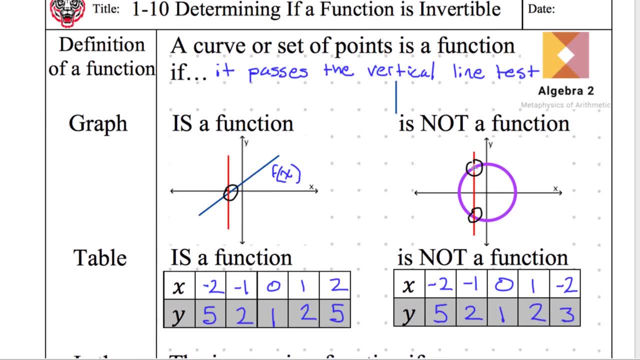 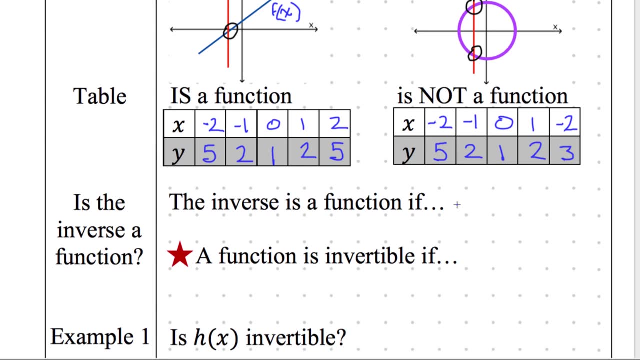 That's why it breaks the function. All right, we're getting to the key material here. The inverse is a function If- And it's basically a throwback to our definition already- If Each X Has only one y. 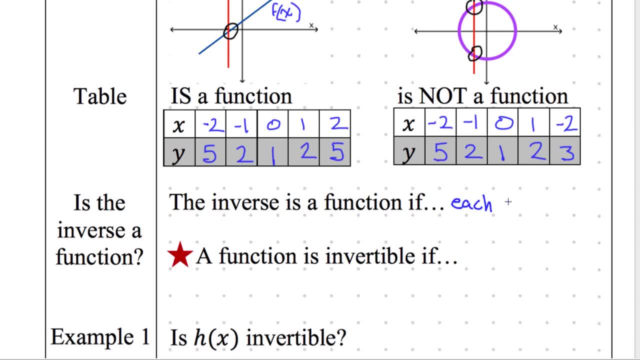 If Each X Has only one y. If Each X Has only one y, Okay, so if one y, If Each X Has only one y, Each input has only one output. I simplified this pretty, like the formal definition in your math textbook would have been. 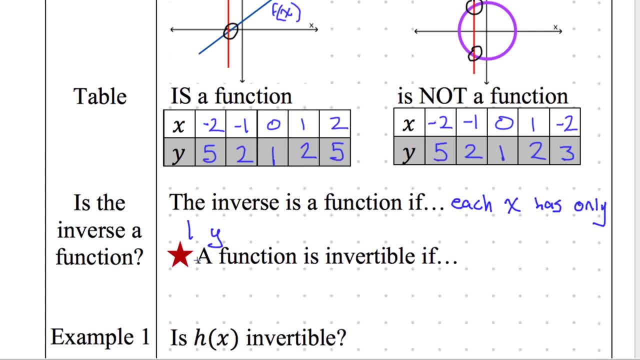 each input has a unique output. I think I simplified it by saying: each x has only one y. That is, check every x, Check every x. That x should have only one y. Well, here's an x and here's an x, but they have different y's. 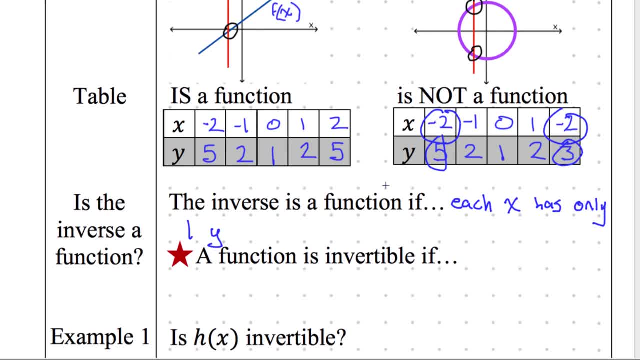 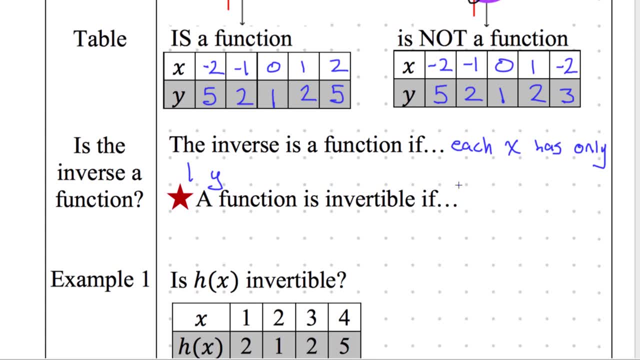 There's two y's for that value of x. That's why I broke that function. I'm just trying to tie everything together, All right, The key part. this needs to be in your summary: A function is invertible if the function has an inverse. 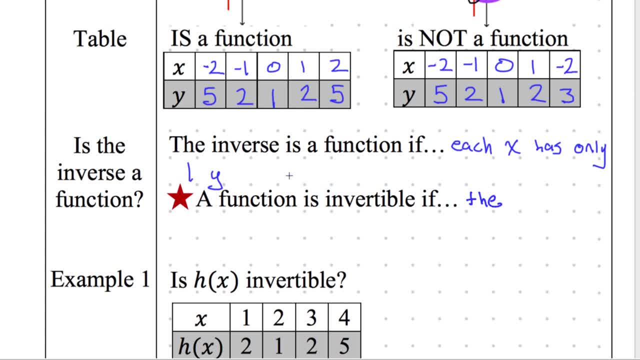 Sorry, that's cyclic. A function is invertible. if you can find an inverse, that is a. That's correct. If the inverse is a function, So find the inverse. If it's a function, that means that that function was invertible. 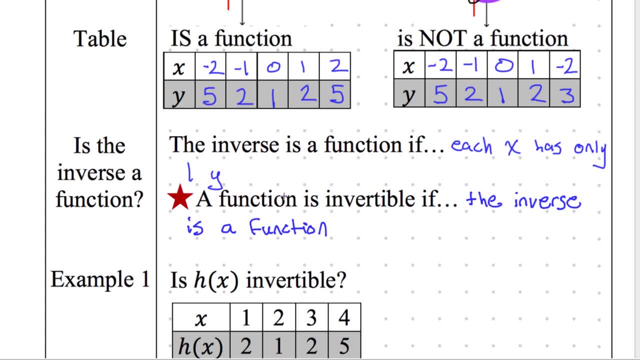 So you're always finding the inverse. You know how to find the inverse. now Check if that inverse is a function. Check if it passes the vertical line test. If it does, then it's invertible. So it's a new keyword here. 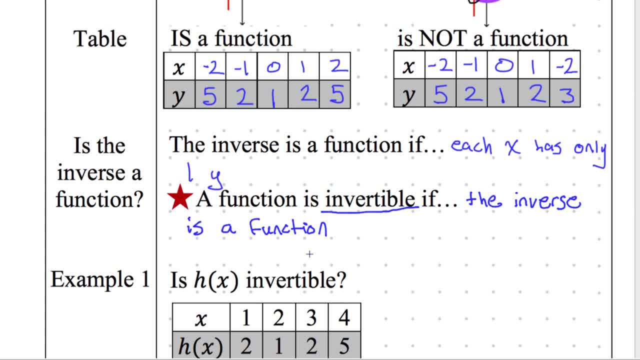 Let's go ahead and just underline it: Invertible. I'm going to be using this for the rest of the unit. Whenever I ask: is it invertible? in your head, you need to be thinking: all right, I'm going to take the inverse and check if it passes the vertical line test. 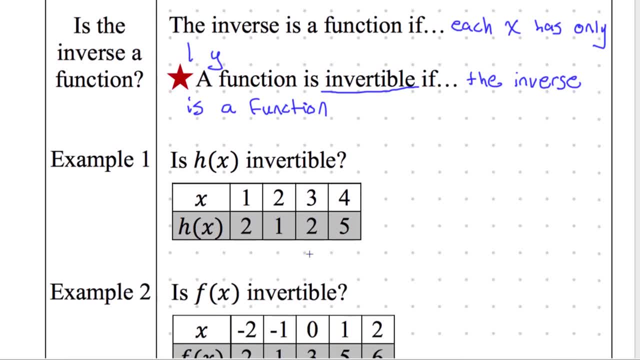 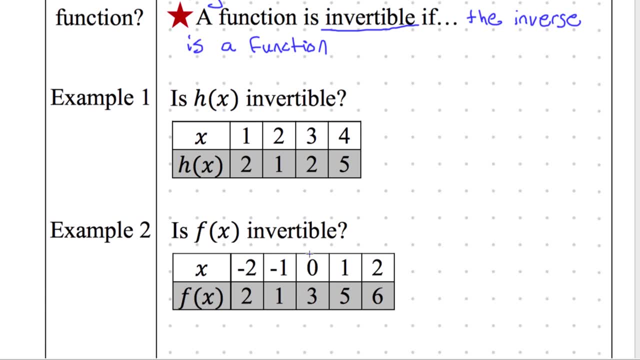 Those are your immediate thoughts. Invertible- All right, Let's check example one: Is this function invertible? So James says yes. What does everyone else say? I want to see thumbs on this one. Just take a guess: Is this function invertible? 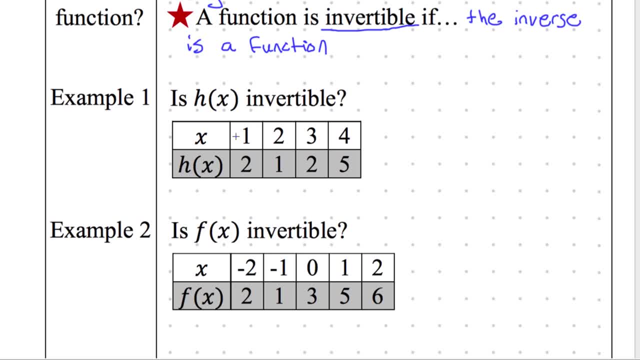 Check each x. If there are duplicate x's, they should go to the same value. If there are duplicate x's that go to different values, you're in trouble. And that's just talking about a function If it's invertible as a different can of worms. I see a lot of yeses. 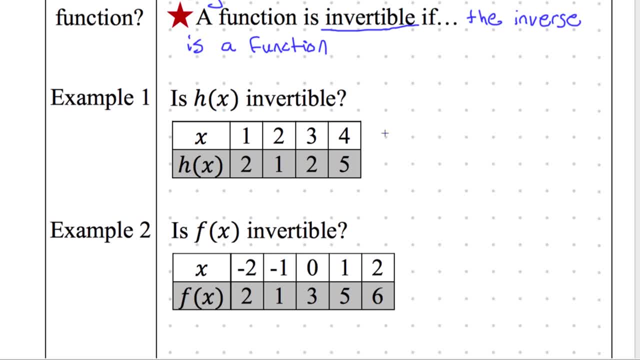 All right. Well, let's take the inverse. The inverse will go this way: The inverse will have xh to the negative 1 of x. You're making a new table out here. Here's the inverse Inverse. How do I find the inverse again? 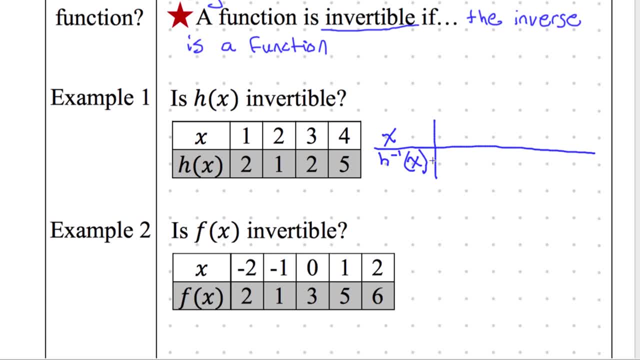 This is a review. You switch, You shout it out. You switch the x and the y. That means, instead of 1, 2,, I'm going to do 2, 1.. Instead of 2, 1,, I'm going to do 1, 2.. 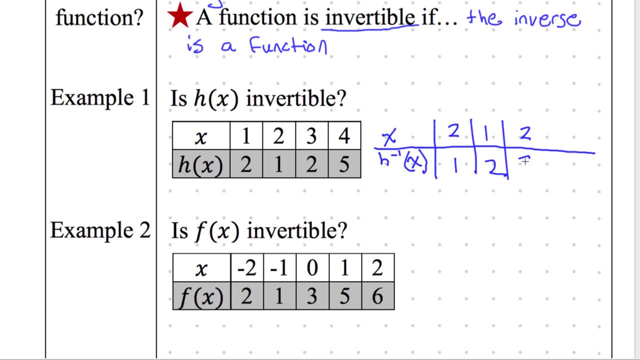 Instead of 3, 2,, I'm going to do 2, 3.. Instead of 4, 5,, I'm going to do 5, 4.. That is the inverse function. I just switched my inputs with my outputs. 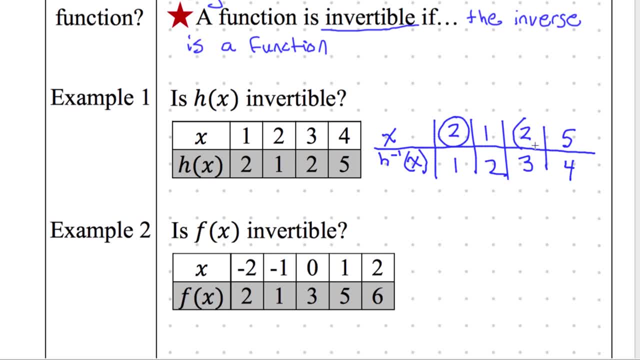 Now I'm going to check For each of my inputs. they should all go to different outputs, But 2, you can see that 2 goes to 1.. 2 also goes to 3.. So I found the inverse. This inverse is not a function. 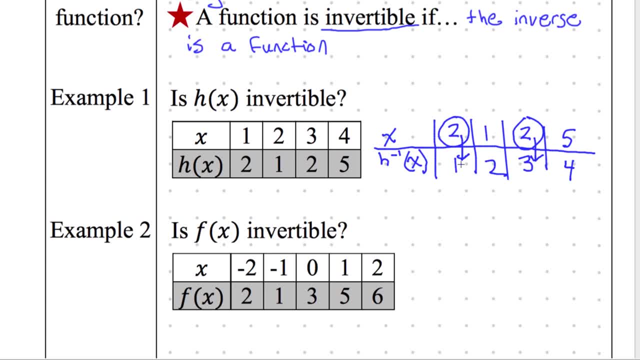 Someone regurgitate back to me. Why is this not a function? Use your own words Or use my words if you can remember them. Why is this inverse function, this x and h to the negative 1 of x, this inverse of h? 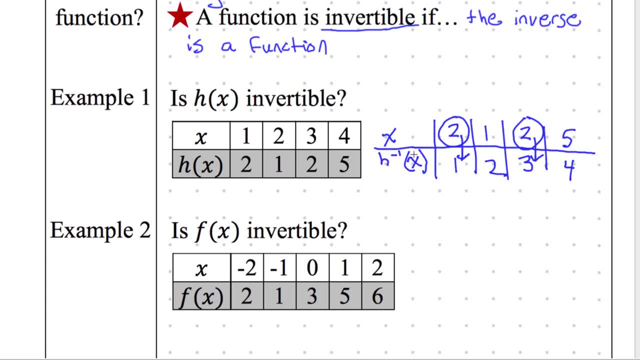 why is this not a function, Andrea? Because the x goes to the same y. Yeah, Say it one more time: Because the x goes to the same y. Yeah, If this one was a 1, it would have been the same y, it would have been okay. 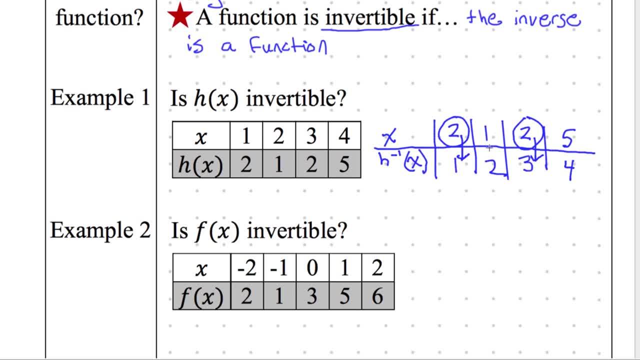 It's just listing that point again. But because the x goes to different y's, it's not a function Perfect. So the answer here is no. Let's try example two, 2 without actually drawing out the table on the right-hand side. Let's try example 2 just by doing. 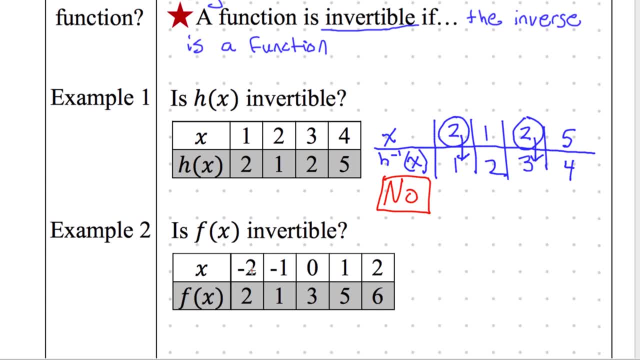 it in our heads. Instead of seeing a negative 2, 2, here see a 2, negative 2.. You just reverse it backwards. Maybe you should, the way that you're visualizing in your head. don't write this down. 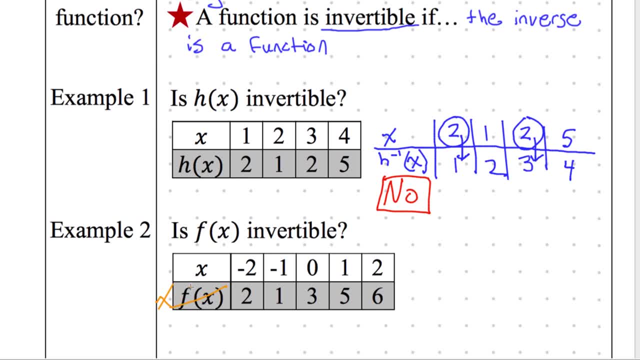 You might visualize this: instead of this being f of x, you can see that's your x. Instead of that being x, that's your f. inverse of x. You're going backwards. now, When you're going backwards, is this f of x invertible? When I find the inverse, is it a function? Does it pass the? 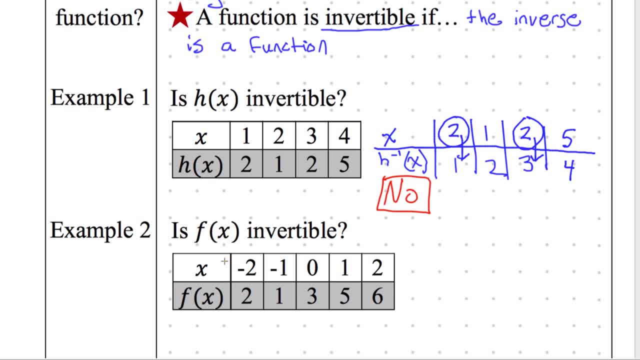 vertical line test. So, going backwards, is it a function? Thumbs up, thumbs down? let's see it. You are all correct, Because b's are now your x values and there's not even a duplicate. If there's no duplicates, it's automatically invertible. 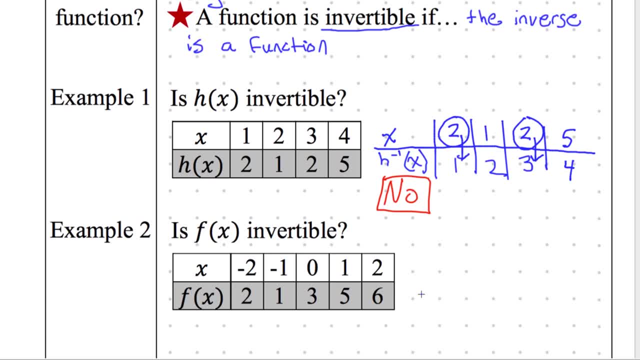 And maybe that's something that you want to write down in your notes. So for down here, no duplicates, And because of that it's yes. And then you check back with example 1.. There were duplicates for h of x, And because those 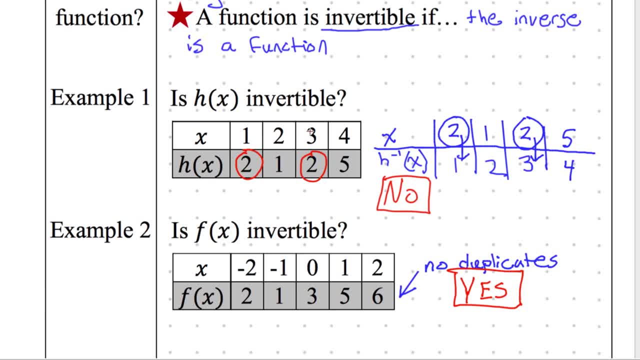 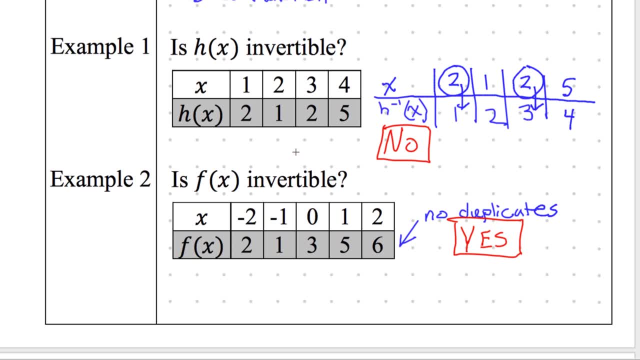 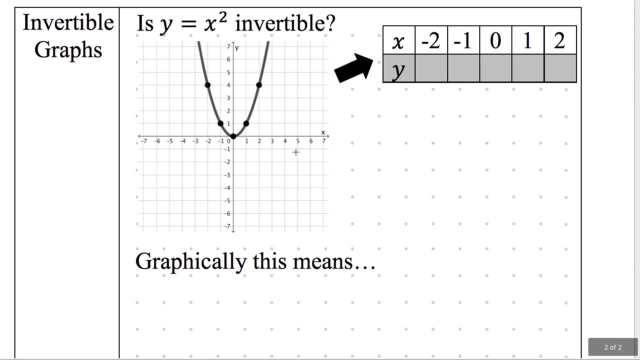 duplicates didn't match up with the same x coordinate. that function was not invertible. All right, Fist to five. how well are you following me so far? So far, so good. okay, thank you. Back side. Now we have to think graphically. 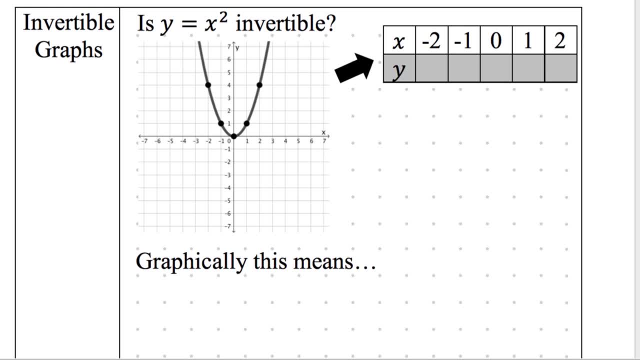 Now you have to think graphically, but we're going to use a table as a crutch, As a scaffold. Is this function- y equals x squared- invertible? Take a guess right now. I just wanna see: Do you think that this function is invertible? 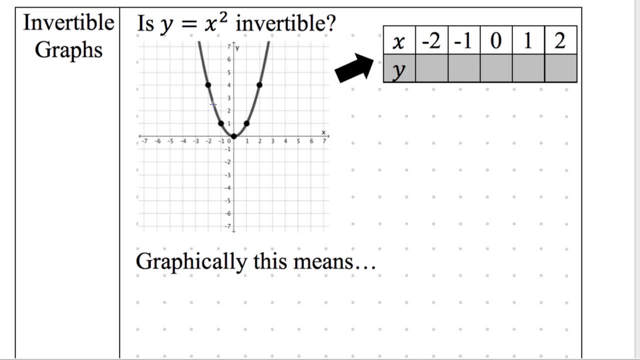 Thumbs up, thumbs down, You still get your XP for trying. I'm going to do it all at the end. Do you think that this parabola, this function of y, equals x squared? do you think, is invertible? Just take a guess: Invertible, Non-invertible. Alright, good guesses. 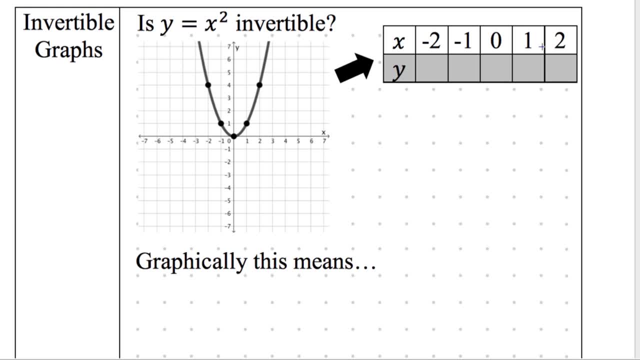 Let's go ahead and make these points that I made on the graph into a table. So negative 2 has a height of. shout it out everyone: Yeah, This x coordinate of negative 1 has a height of. This x coordinate of 0 has a height of. 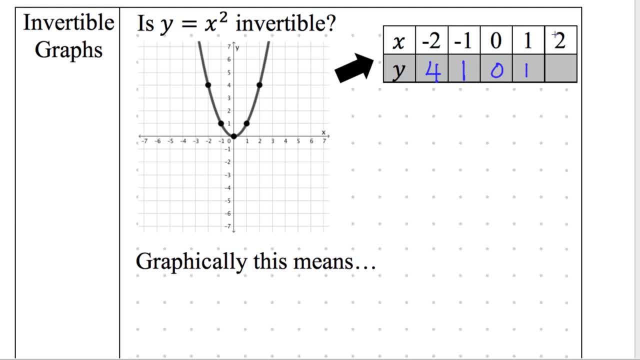 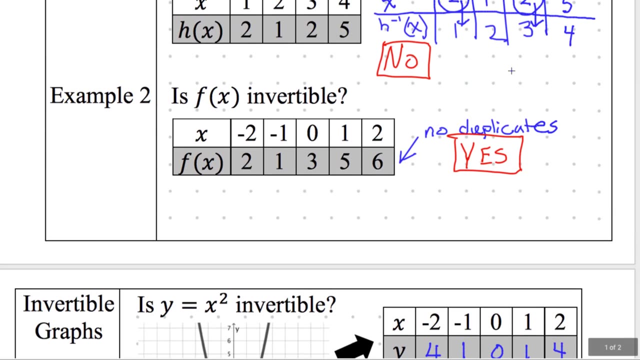 1 goes to 2 goes to Very nice, yeah. Alright, now that you see the table, take another guess. Is this function invertible, Yes or no? Thumbs up, thumbs down. Remember you're asking yourself: are there duplicates down here? 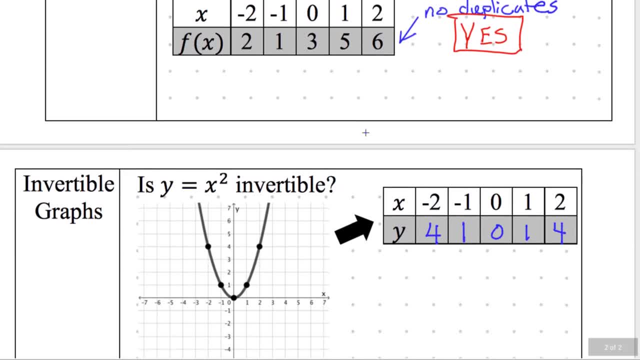 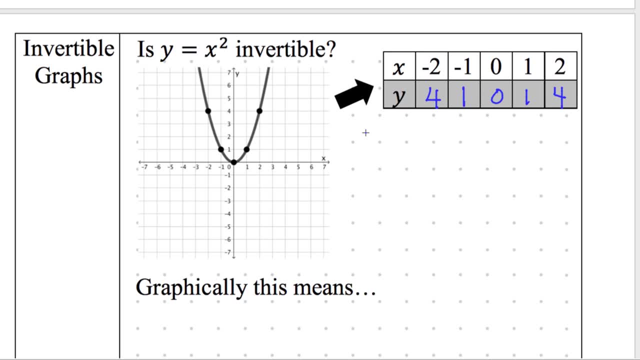 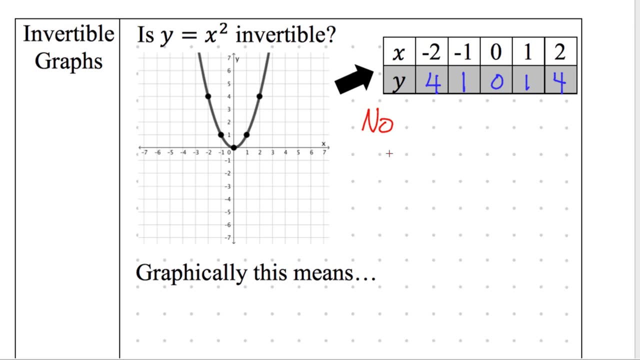 And if there are, do they have matching x coordinates? Thumbs up, thumbs down. I see mostly thumbs down, one thumbs up. So the answer here is no, it's not invertible. No, it's not invertible Because I had duplicates down here and they went to different values up here. 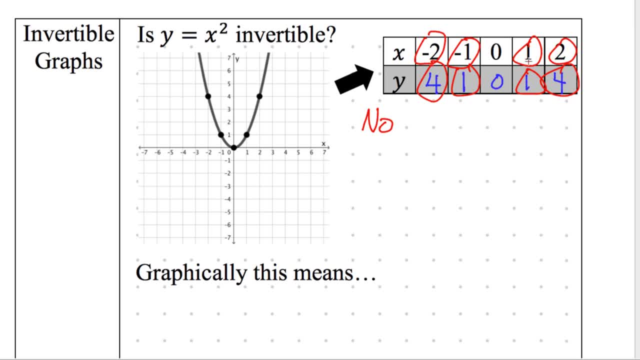 I had duplicates right here. they went to different values up here. There are two ways to disprove that. Ah, so that's a good point. Vertical line test means that this function, y equals x squared, is a function, but is the inverse of that a function is what we're asking now. 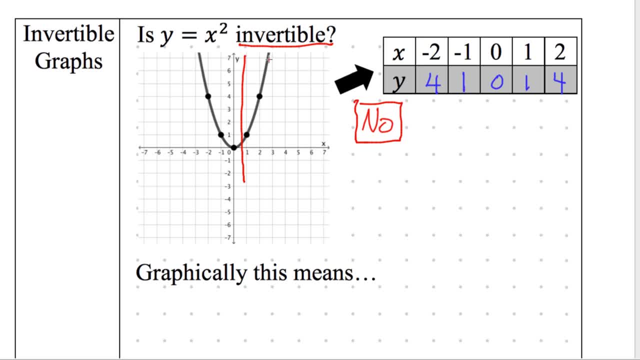 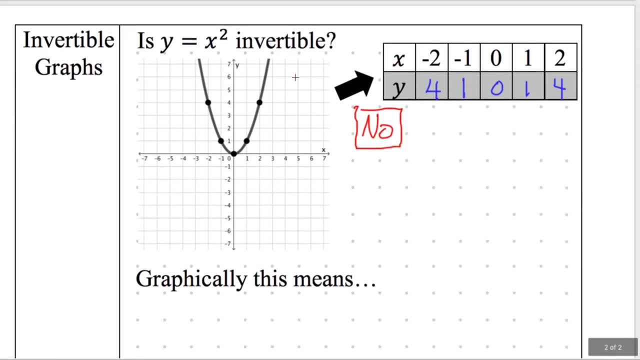 Because that's what invertible means- Is the inverse of this a function. And if you recall from- I think it was lesson- I think it was 1-7,, maybe 1-6, the inverse of this function. if I were to graph it on Desmos, it would look like this: 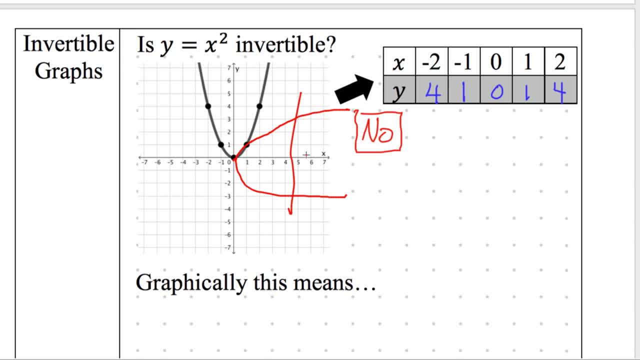 And because of that I have a vertical line test that doesn't pass. therefore, it's not invertible, Because invertible means you're reflecting over this line. y equals x. This is pretty cool graphically too. You can do this graphically without converting to a table. 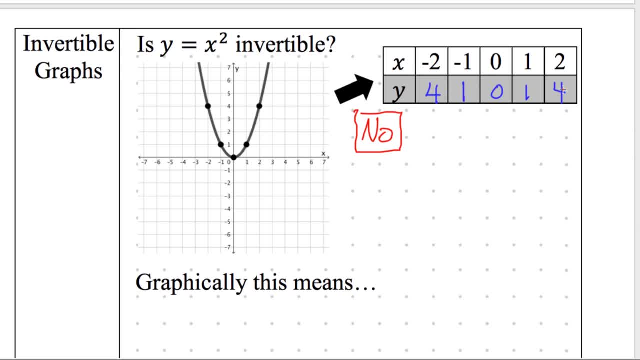 That means that if I look at this height of 4 and 4, this height of 4 and 4, that is represented by a horizontal line, This horizontal line right here. Notice that I said if there were duplicates for the height and they went to different values. 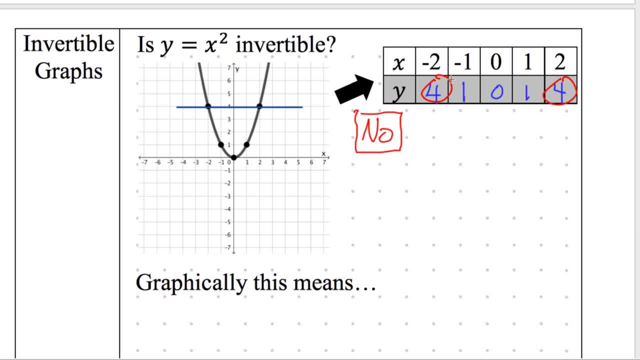 that means it's not invertible. Graphically that means with this height of 4 and 4, this line right here, if it passes through two different x-coordinates, it is not invertible. Now we have a horizontal line test to tell if a function is invertible. 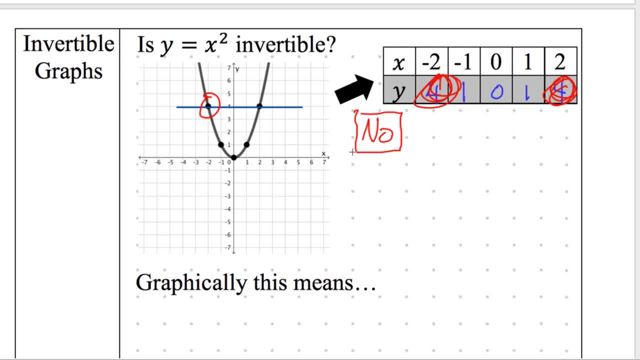 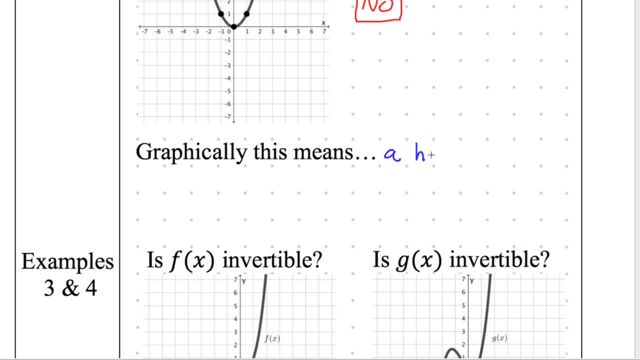 A horizontal line test to check if it's invertible. So let's go ahead and undo all that scribbling and write it down Graphically. this means a horizontal. a horizontal line can only pass through the curve once, one time.